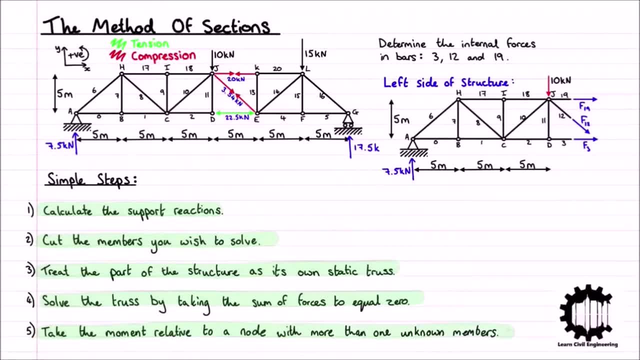 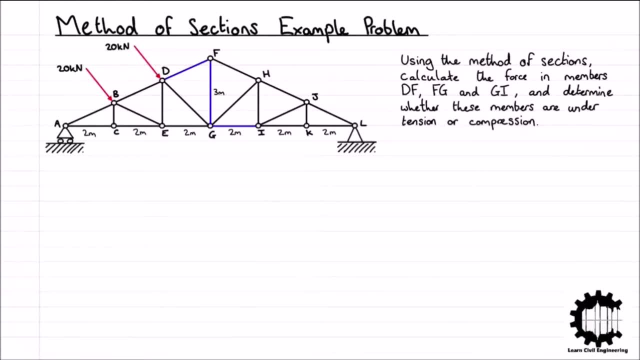 and finally, we take the moment relative to a node with more than one unknown members. With that summary, we will begin to solve our example problem. We have a roof structure which is in the shape of a Howell truss, supported by a roller at node A and a pin support at node L. 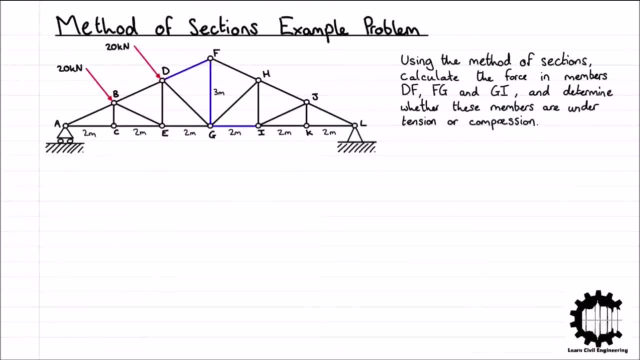 All the horizontal members of the truss are 2m in length and the vertical members are 1m, 2m and 3m in length, from the outer to the inner members respectively. We also have external loads of 20kN being applied to node B and node D. 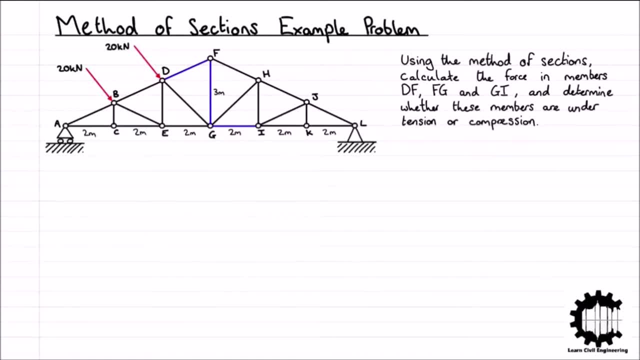 which are acting on the structure perpendicularly. Thus we arrive at the solution of the problem. We have two different forces, the ones which we need to solve, and each of these two forces are subject to the line AF. Using the method of sections, we must calculate the forces in members: DF, FG and GI. 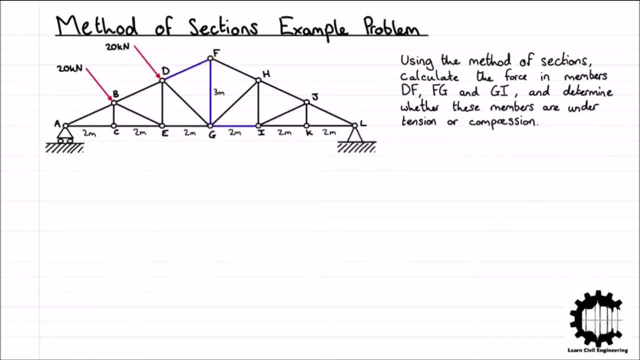 and determine whether each of these members are being subject to tension or compression, and you're welcome to pause the video here to attempt this question for yourself. So now let's get into the solution. Before we begin to solve any of the forces, there are a couple of things we can do to help us with. 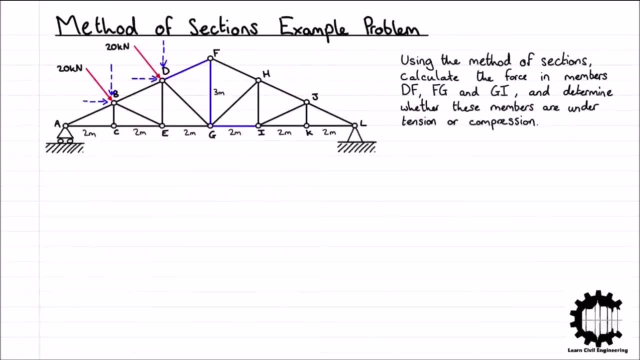 the rest of the problem, components of the forces being applied to the structure and generally. I'd recommend doing this for most questions within structural analysis, as they greatly simplify the following steps. First of all, we can acknowledge that we can use the concept of similar shapes to simplify. 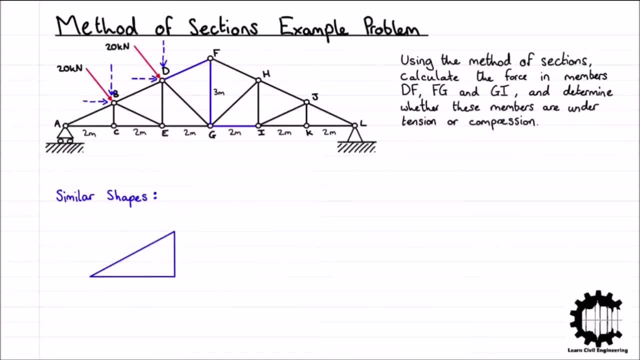 the external loads. Similar shapes are shapes of the same proportion and so can become identical after being scaled, rotated or flipped. Here we can see that the right angle triangle with a width of 2 metres and a height of 1 metre can be scaled and rotated to help us find the horizontal and vertical components. 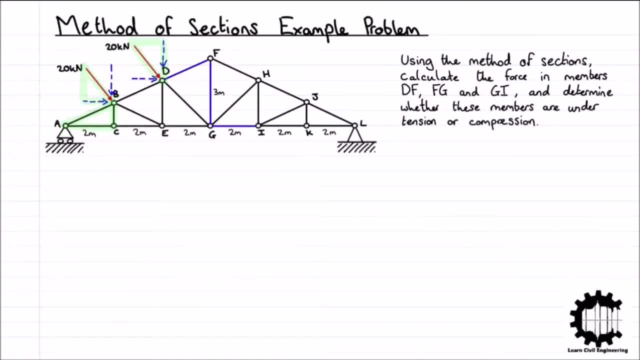 of the 20kN external forces. The horizontal and vertical components of the external forces will be needed for resolving the horizontal and vertical forces later on. so let's work out these components, To start with, a horizontal length of 2 metres and a vertical length of 1 metre, using Pythagoras. 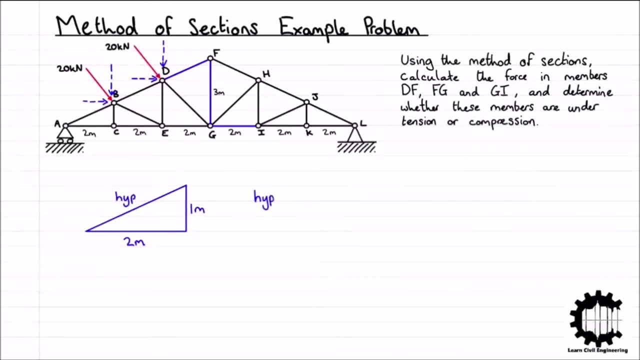 theorem, we can calculate that the length of the hypotenuse of the triangle is equal to the square root of 2 squared plus 1 squared. This equals the square root of 5 metres. Now for the horizontal component of the external forces. we have the external force of 20kN. 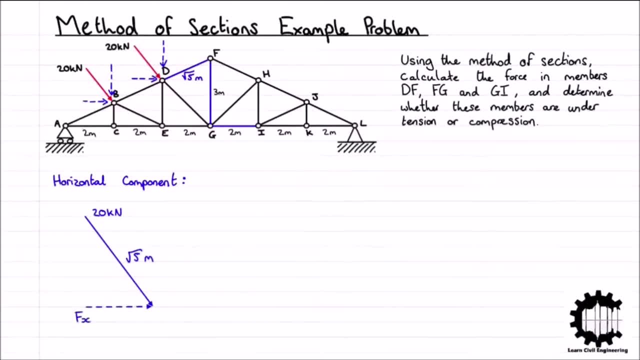 over a length of root, 5 metres, and we have the horizontal component, Fx, over a length of 1 metre, with the angle between the external force and the vertical plane being theta. Therefore, Fx is the opposite side of the triangle and the external force is the hypotenuse. 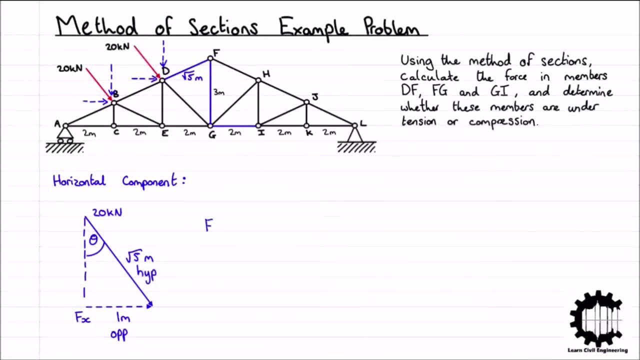 of the triangle. Using trigonometry, we can work out that Fx is equal to 20kN times sine theta, where sine theta is equal to the opposite over the hypotenuse, which equals 1 over the square root of 5.. Therefore, the 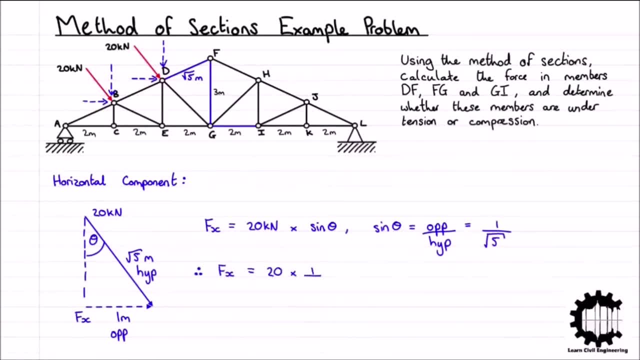 horizontal component of the external force Fx equals 20 times 1 over root 5, which equals 8.944kN to 3 decimal places. Now, doing the same for the vertical component, we have the external force of 20kN over a length of root 5m and we have the vertical component Fy. 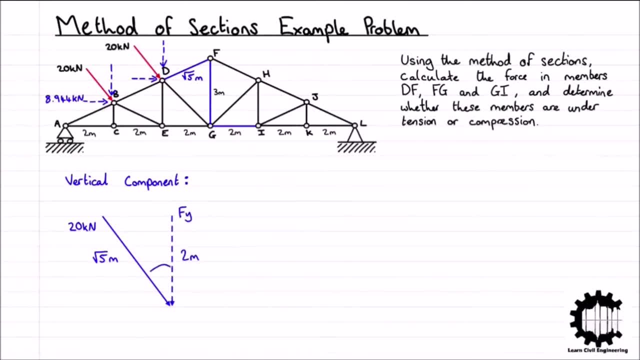 over a length of 2m, with the angle between the external force and the vertical plane still being theta. Therefore, Fy is the adjacent side of the triangle and the external force is the hypotenuse of the triangle. Using trigonometry, we can work out that Fy is equal. 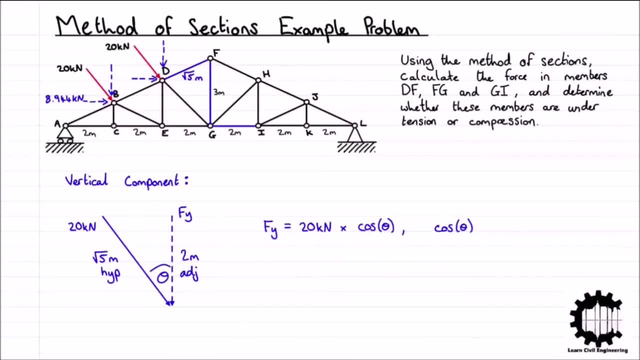 to 20kN times cos theta, where cos theta is equal to the adjacent over the hypotenuse, which equals 1 over the square root of 5.944kN. Therefore, the vertical component of the external force Fy equals 20 times 2 over root 5, which. 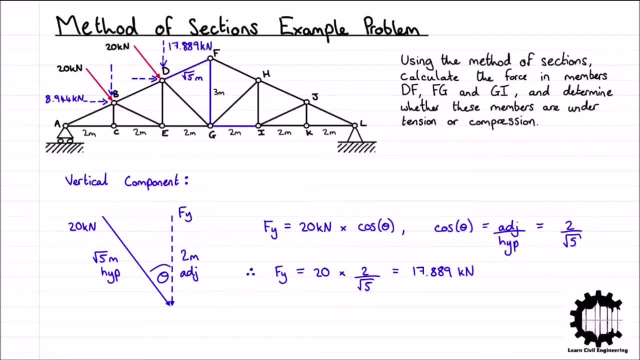 equals 17.889kN to 3 decimal places. Having determined the horizontal and vertical components of the external forces, we can start to work out the forces in the required members. We will need to work out the reaction forces at the supports Rav, Rlv and Rlh. 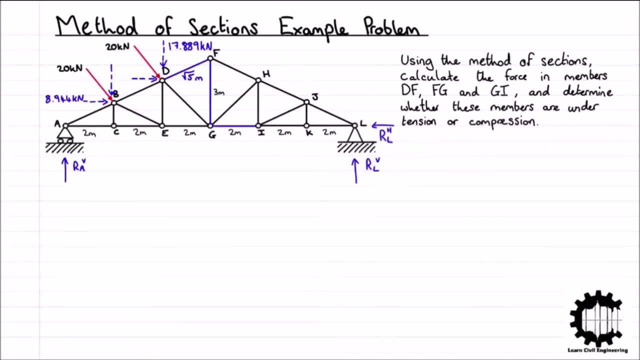 but before we do that, let's see where we will make our cut. to divide the structure into two substructures, We have to find the internal forces in members dF, Fg and Gi. so we will cut our structure through members dF, Fg, Gh and Gi, like so. 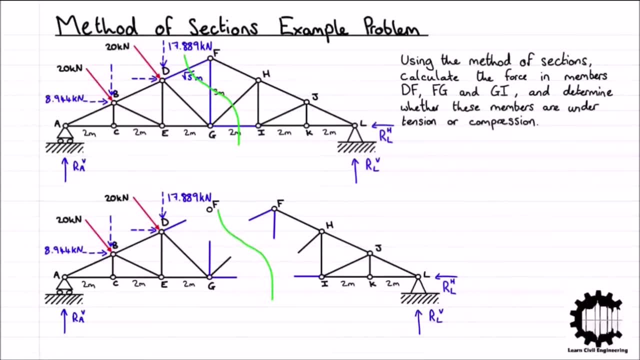 and this leaves us with two separate trusses, which we will consider as independent structures from now on. For this example problem, we will only consider the left-hand structure, so we only need to determine the change in the reaction force at node A before we can discard the right-hand structure. 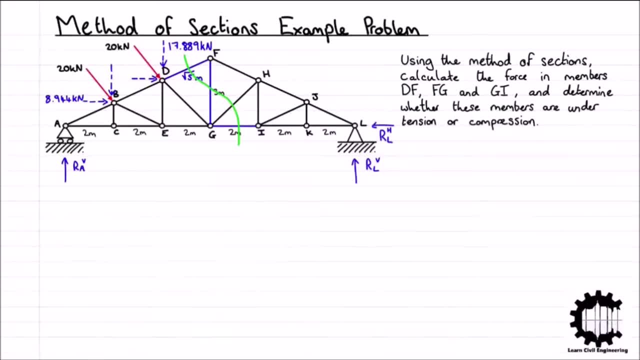 To calculate RAV, we will consider the entire structure, taking the moments about node L, as this eliminates all unknowns from the equation except for RAV. As the structure is in equilibrium, the sum of all moments about a point must be equal. 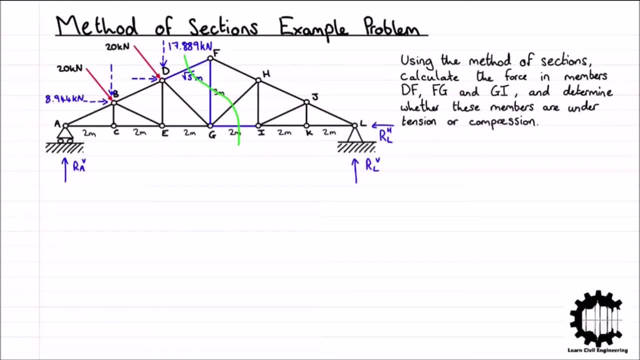 to zero. So, taking the anticlockwise rotation direction to be positive, the sum of moments about node L is equal to 12RAV plus 1 times 8.944 plus 2 times 8.944 minus 10 times 17.899 minus. 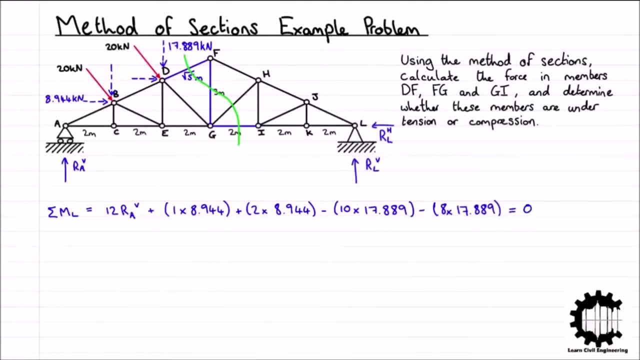 8 times 17.899, which equals zero. Rearranging this equation for RAV and then solving, we get that RAV is equal to 24.598 kN, to three decimal places. Having calculated the support reaction force at node A. 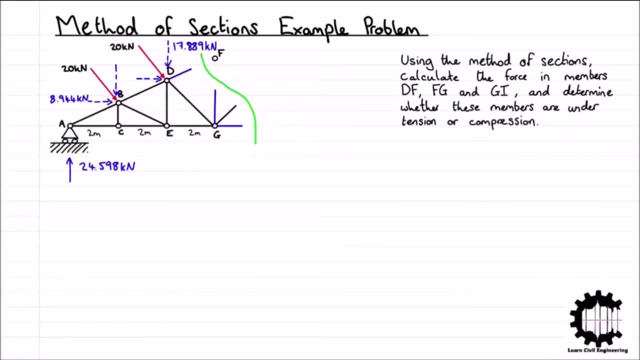 we can now add the support reaction force at node B. We can now apply our cut to the entire structure and discard the right-hand side, leaving us with this. In order for our structure to remain in equilibrium, we must replace the cut bars with the internal. 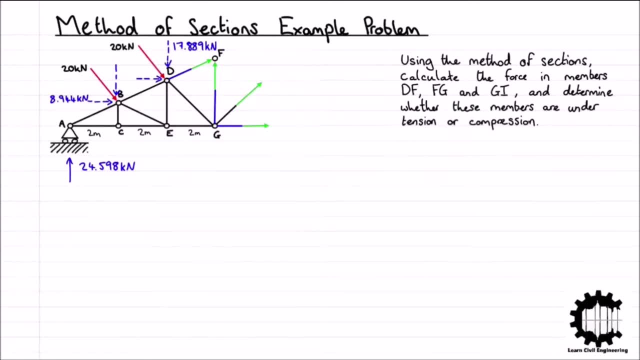 forces, as these will stabilize the support reaction, and external forces being applied to the structure. Doing so, we have internal forces- FDF, FFG, FGH and FGI like so Note here that we are assuming the sensors of the internal forces to be tentative. 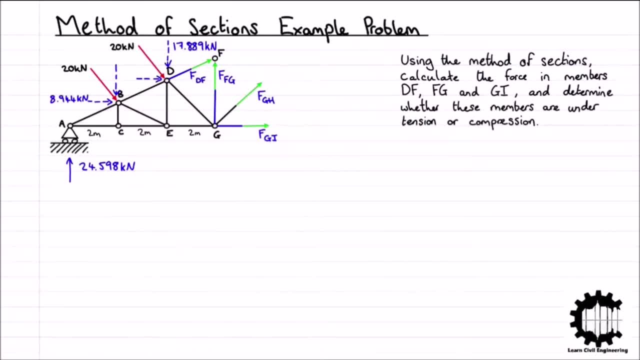 We must ensure that they are not tensile, as they all originate from the centers of the cut bars and are acting in the direction towards the end of members. Before we go on to the sum of the moments about any of the nodes we are going to identify, 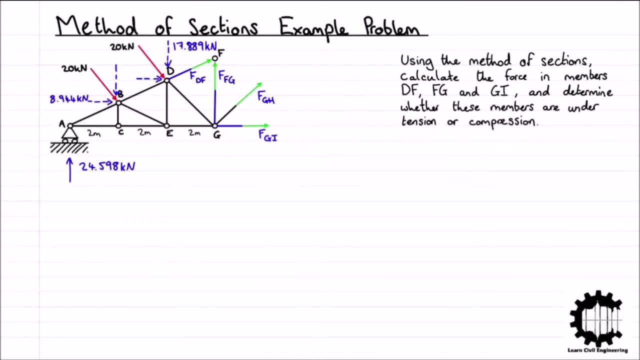 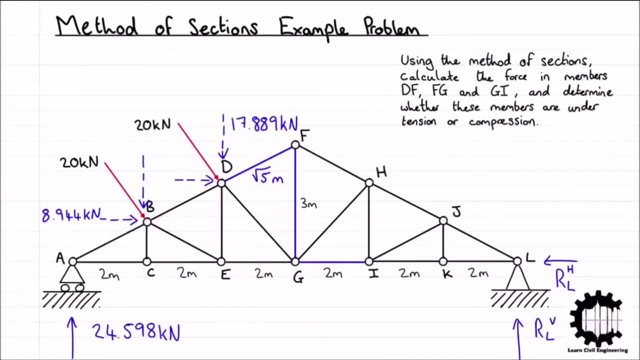 which members in the truss have internal forces of zero magnitude. We will do this by inspection. To do so, we will temporarily consider the entire structure again, Starting by considering node K. for it to be in equilibrium, all forces applied to the members attached must sum to equal zero. To do so, we will temporarily consider the entire structure again, Starting by considering node K. for it to be in equilibrium, all forces applied to the members attached must sum to equal zero. Let's hope the results are satisfactory. 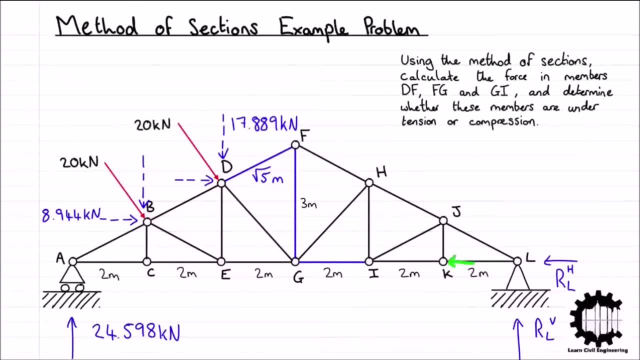 All forces applied to the members taken must be summed to equal zero. If it is not, then we have reached the right balance. If there is a tensile force in member KL, there must be an equal and opposite force to balance it out. 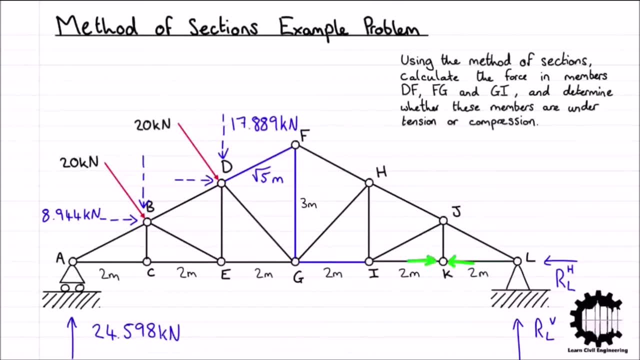 And so there would be a tensile force in member IK of equal magnitude. Now let's say there was a tensile force in member JK. Again, we need an equal and opposite force to balance it out. However, we can see that there are no members attached to node K that would allow this. 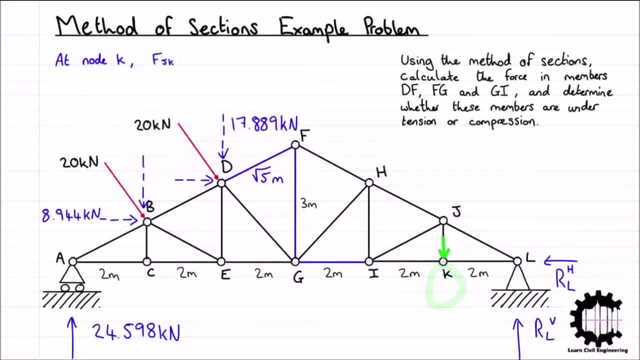 So, therefore, the internal force in member JK must have a magnitude of zero. We will now apply this logic as we work through the structure At node J. an internal force in member JL can be balanced out by an equal and opposite force in member HJ. 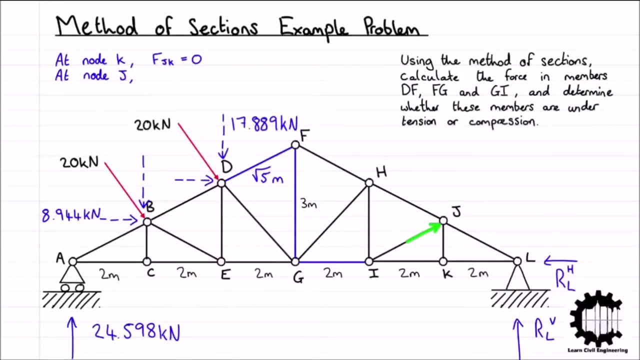 However, with the internal force in JK equaling zero, there are no other members attached to node J that could balance out an internal force in member IJ. So member IJ has an internal force of magnitude zero. At node I, an internal force in member IK can be balanced out by an equal and opposite force in member IJ. 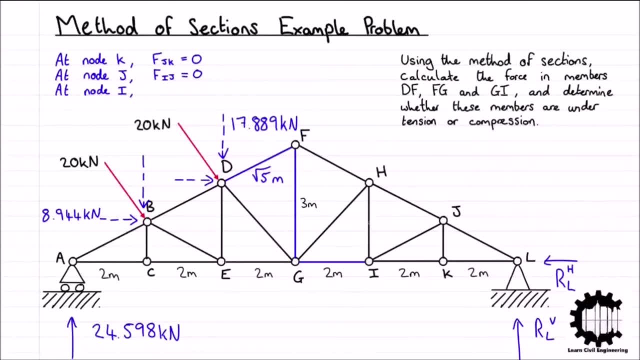 Also, we can see that there is an internal force in node GH equaling zero over node IJ and also there is an internal force in nodeấtal. Floorout from this phenomena, the internal force in HH can be balanced out by an equal and opposite force in node FH. 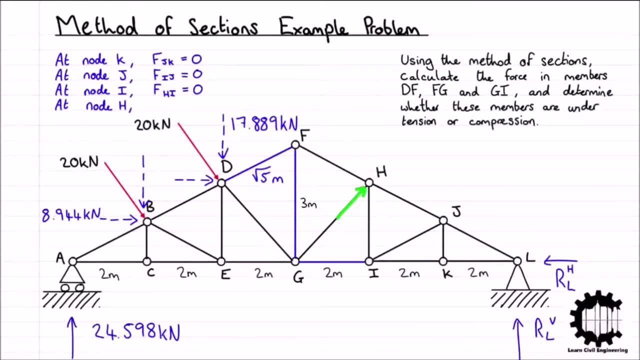 riceая. Finally, if we look at node H, an internal force in member HJ is equal and opposite force in member FH to node H. that could balance out an internal force in member GH. so member GH has an internal force of magnitude zero. And notice here that we have just solved our first unknown, which 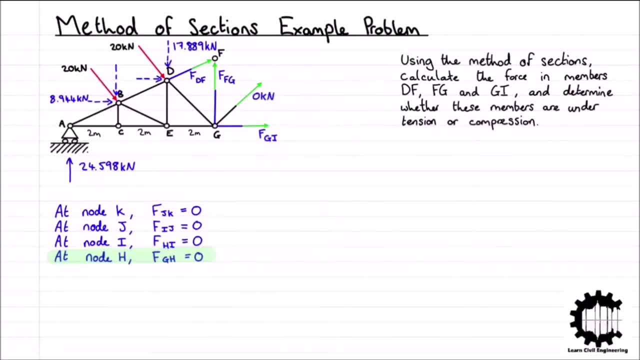 will make solving the rest of our problem a lot easier. Going back to the left side of our structure, then we will determine force FDF by equating all moments about node G to equal zero. We have chosen this node to start, as it eliminates. 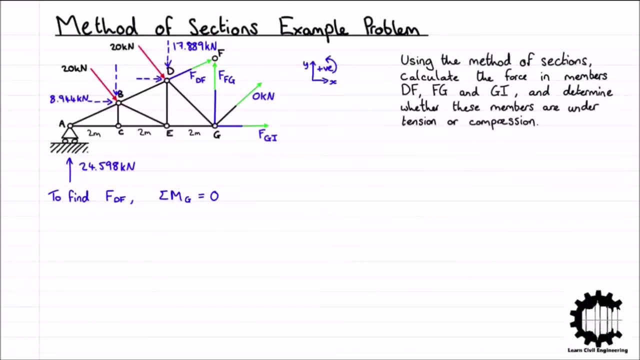 the other unknowns from our equation. So, taking the anticlockwise rotation direction to be positive, the sum of all moments about node G equals negative 24.598 times 6, plus 17.889 times 4 plus 2, minus 8.944 times 1 plus 2, minus 6 over root, 5 times FDF, which 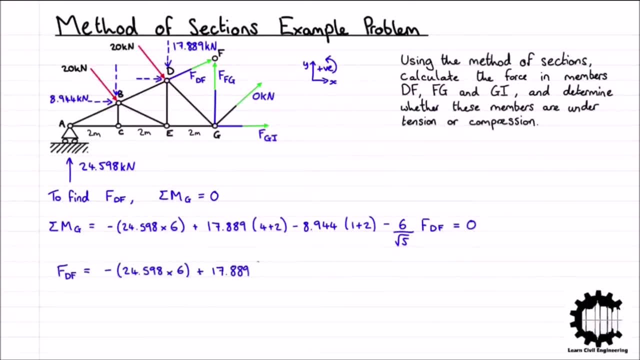 is equal to zero Rearranging for FDF and solving we get. FDF equals negative 25 kilonewtons For member DF. as we assume the internal force to be tensile and our value for FDF is negative, the force of 25 kilonewtons in member DF is: 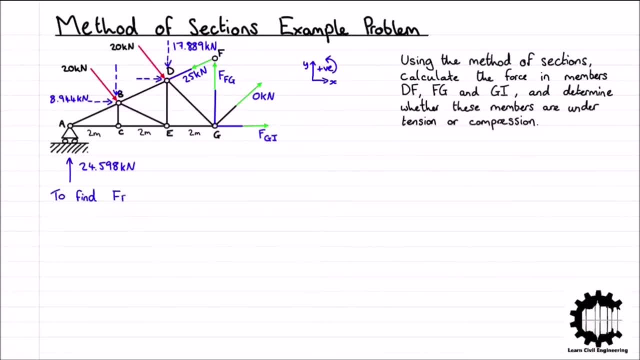 compressive. Now to solve the internal force in member FG. we will repeat this process, taking the moments about node A to equal zero, as this eliminates unknown FGI from the equation, Taking the anticlockwise rotation direction to be positive. the sum of all moments about 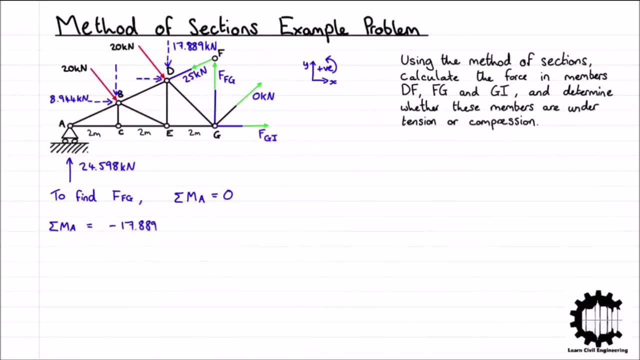 node A equals negative 17.889 times 2 plus 4, minus 8.944 times 1 plus 2, plus 6, FFG, which is equal to zero. Rearranging for FFG and solving we get FFG is equal to 22.36 kilonewtons and, as we assumed, the internal force in member FG. 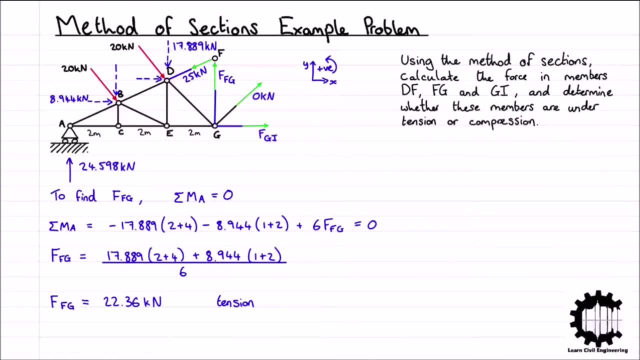 to be tensile and our value for FFG is positive. the force of 23.36 kilonewtons is equal to 22.36 kilonewtons. Finally, to solve the internal force in member GI, we will take the moments about node F. 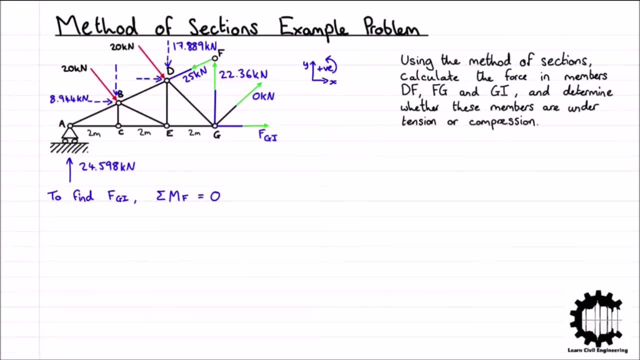 to equal zero For the last time, taking the anticlockwise rotation direction to be positive, the sum of all moments about node F is equal to 17.889 times 4 plus 2, plus 8.944 times 2 plus 1,. 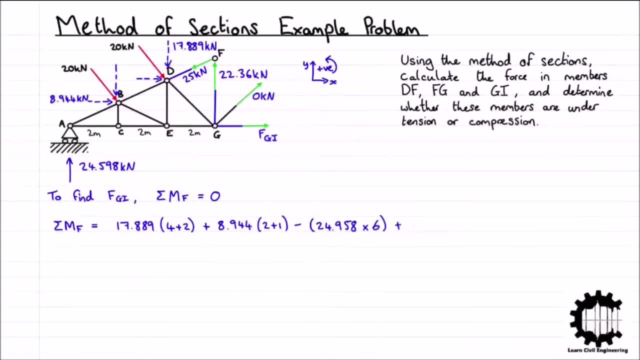 minus 24.958 times 6, plus 3 times 6.. Finally, to solve the internal force in member GI, we will take the moments about node F to equal zero For the last time, taking the anticlockwise rotation direction to be positive the sum. of all moments about node F is equal to 23.36 kilonewtons and, as we assumed the internal force in member GI to be tensile and our value for FFG is positive, the force of 23.36 kilonewtons is equal to 22.989 times 4 plus 2, plus 8.944 times 3 times FGI, which is 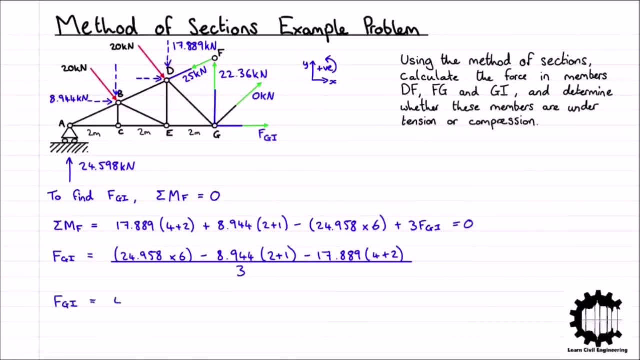 equal to zero. Rearranging for FGI and solving we get FGI is equal to 4.47 kilonewtons and, as we assumed the internal force in member GI to be tensile and our value for FGI is positive, the force of 4.47 kilonewtons in member GI.